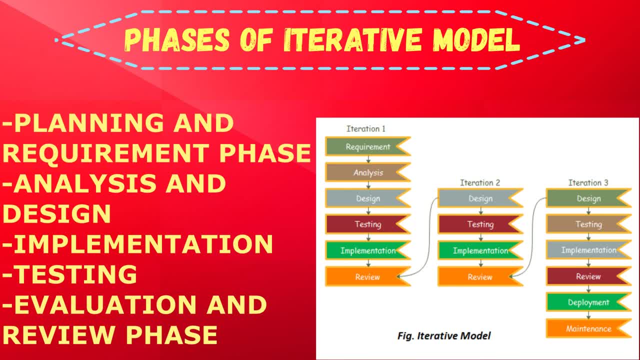 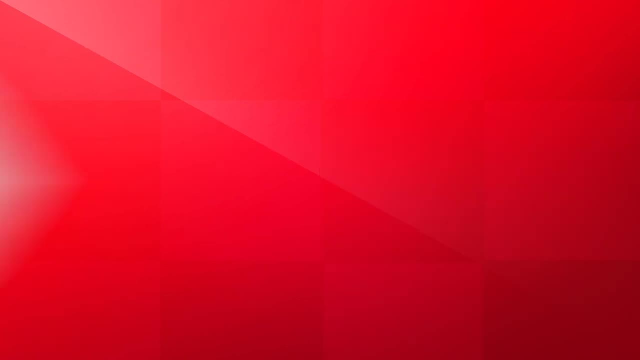 The second one is of analysis and design phase. Third is of implementation phase, Fourth is testing phase And the fifth one is evaluation and review phase. So these all are the phases which is include inside the iterative model. Now we are going to see in details of each phase. Now we 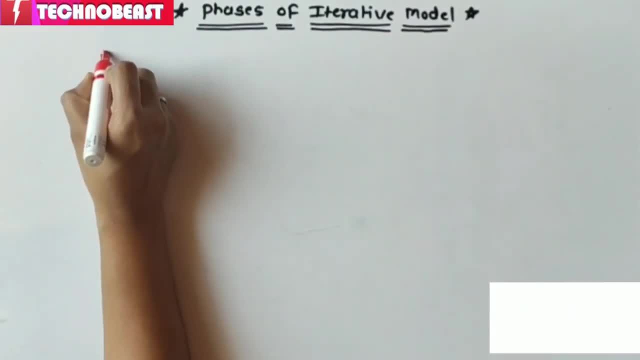 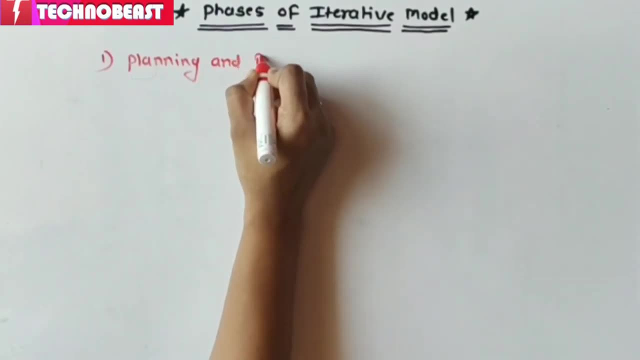 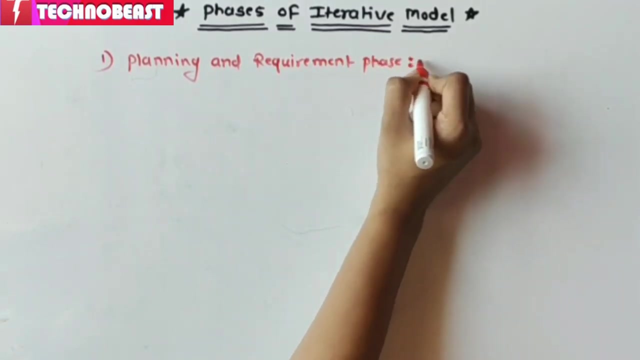 are going to see the phases of iterative model, in which the first one is planning and requirement phase. So this is the first phase of this iterative model, that is, planning and requirement phase. Okay, so, as we know that it is a first stage of iterative model and every first stage will first 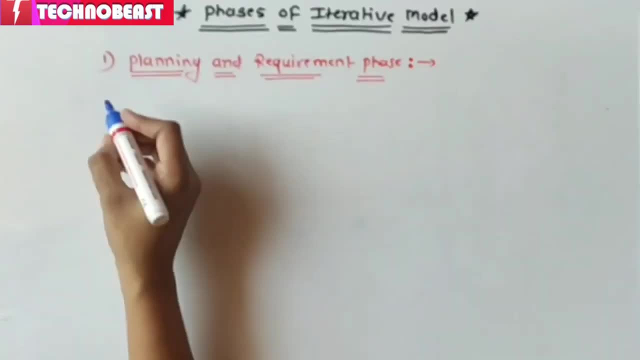 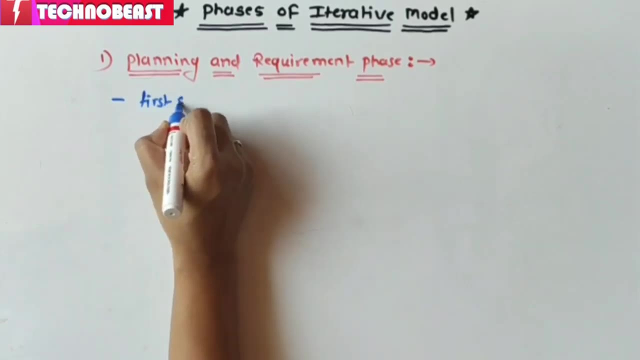 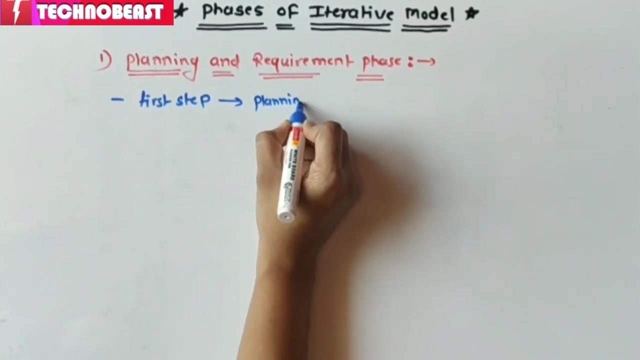 gather the information or requirement from the client. So, as with the most any development project, the first step is planning and requirement phase. So, as we know that it is a first stage of is go through the initial planning stage means we are first going through the initial planning. 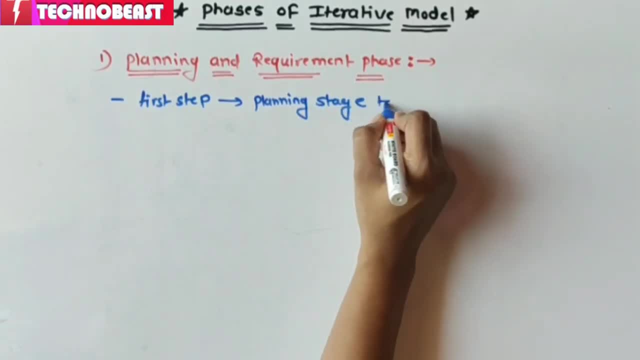 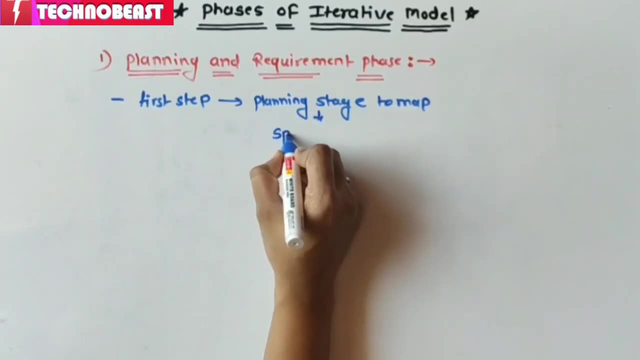 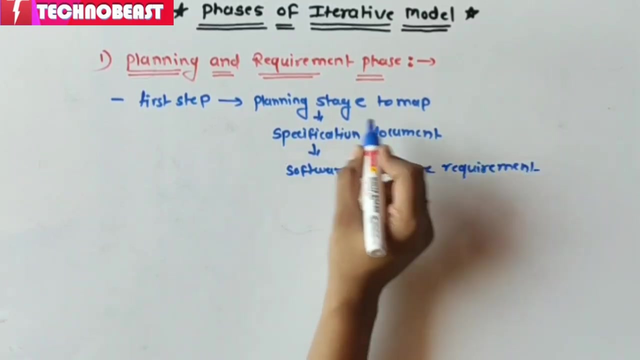 stage. uh, for what to map out? okay, what we have to do to map out the specification document. by using this, we are mapping out these specification documents and that okay. so, with the help of specification document, we are establishing the software and hardware requirements- right, software or hardware requirements with the help of these specification document. okay, 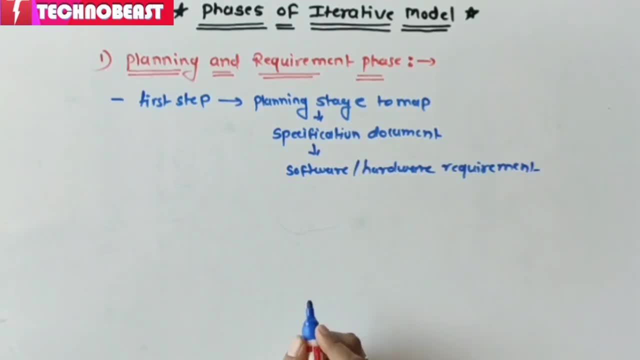 so generally prepared for this upcoming stages of this cycle we are doing for the upcoming stages means planning and requirement phase. okay, in this requirement phase the software development, the system related information is gathered and analyzed. means, here the system related information is gathered and analyzed. means firstly, in requirement phase we 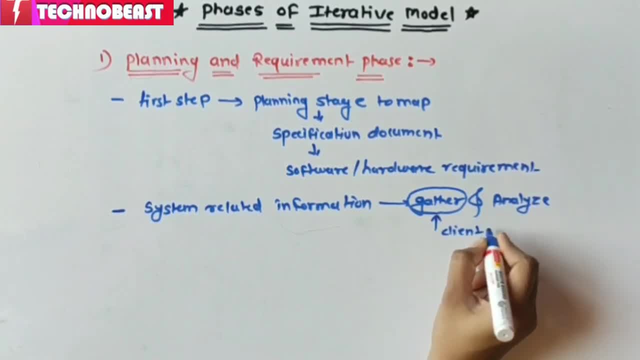 are gathering the information from client, or we can say that user, and then, after gathering all these documents, or we can say that all requirements we are going to analyze them, that collected requirements are then planned accordingly for the development of the system means whatever we are gathered and analyzed according to that, we are planning for the. 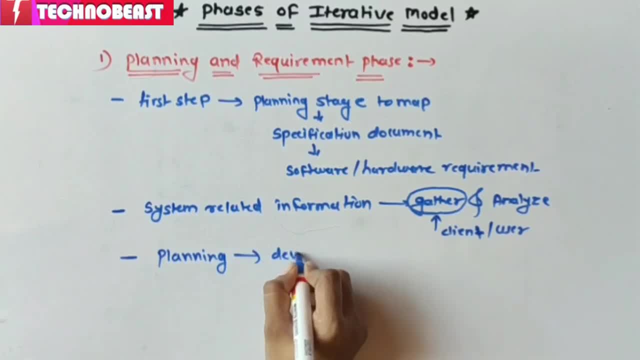 develop the system right. so here this is all about the planning and requirement phase, as, firstly, we are gathering the information from the client right. so with the help of this gathering information will making document right and with the help of that documents we are going to plan to develop the system. so these all are the things happen inside the first stage, that 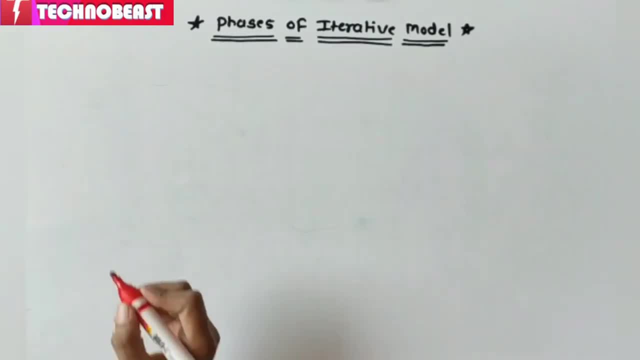 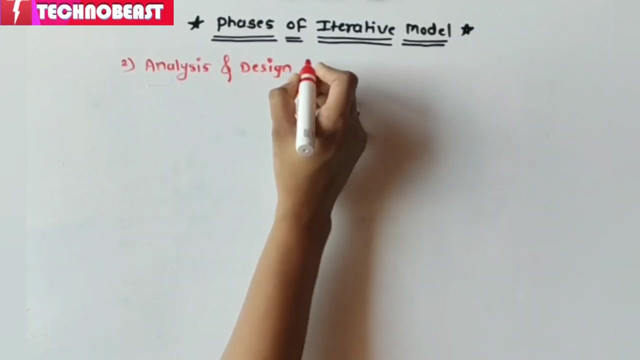 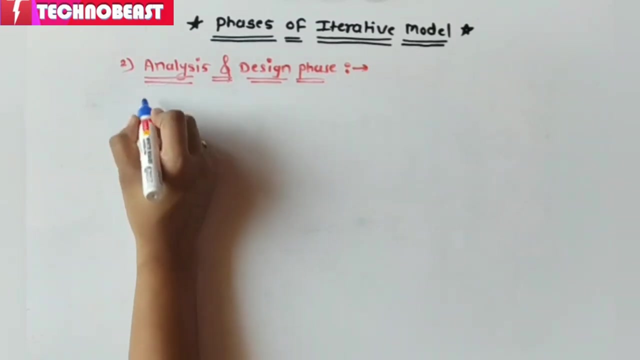 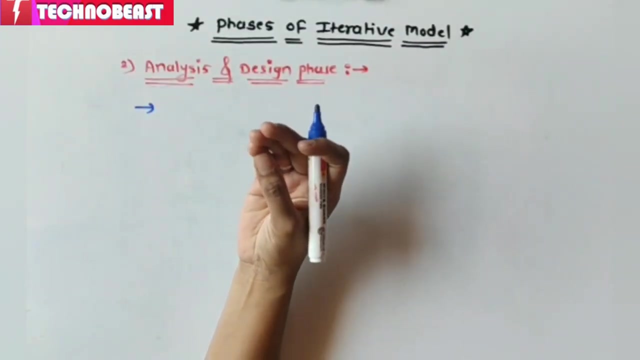 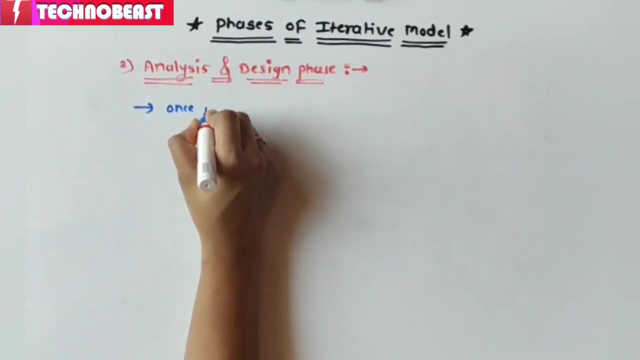 is planning and requirement phase. okay, now we are going to see our second phase, that is, of analysis and design phase. in this analysis and design phase, will planning something to do, a complete process to do? a complete process Means once a planning is complete. here an analysis is performed to nail down the appropriate business logic. Means here, once we have to complete our planning right. 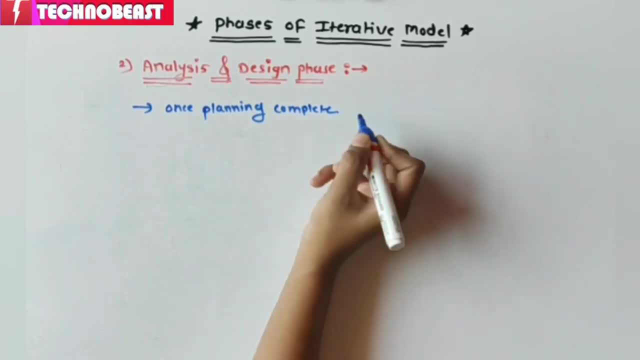 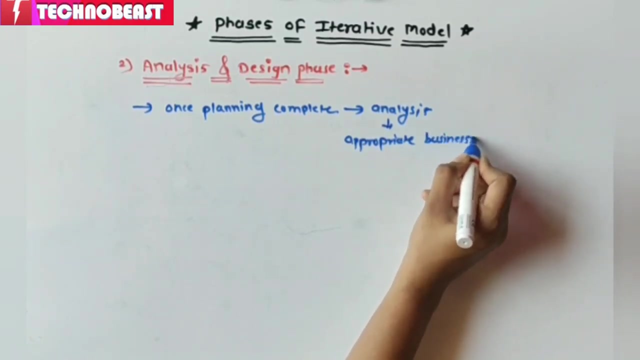 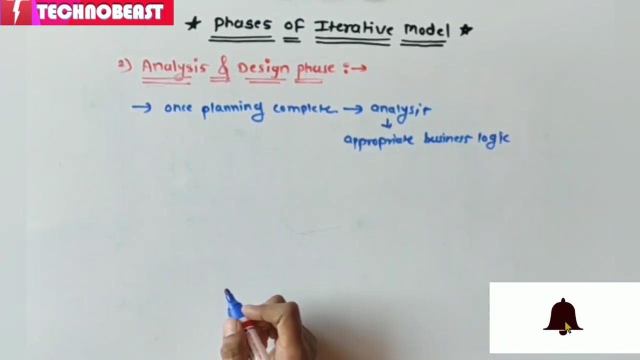 So, once planning is complete, we are going to do the analysis, to perform, nail down the appropriate business logic. Appropriate business logic means what we have to do in the project, that we have to decide in this analysis path And the database models and like that will be required at this stage in this analysis. 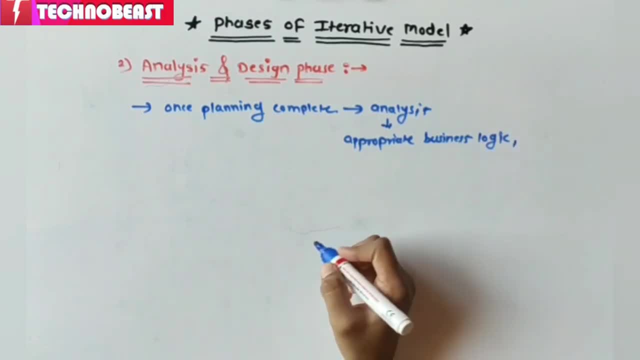 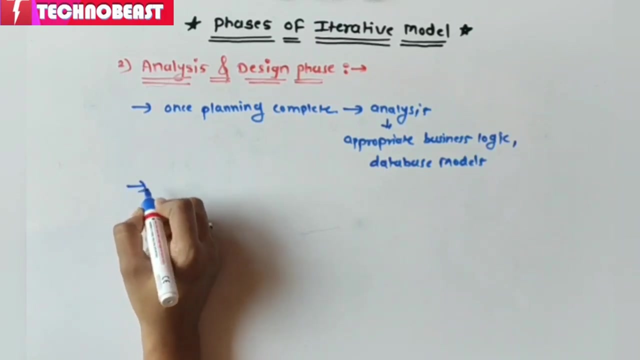 Project means appropriate business logics, or we can say that which database model we have to use, that will be decided in this analysis phase. Means analysis and design phase. The design stage also occurs here. establish any technical requirements. right Here we are also deciding the technical requirements. 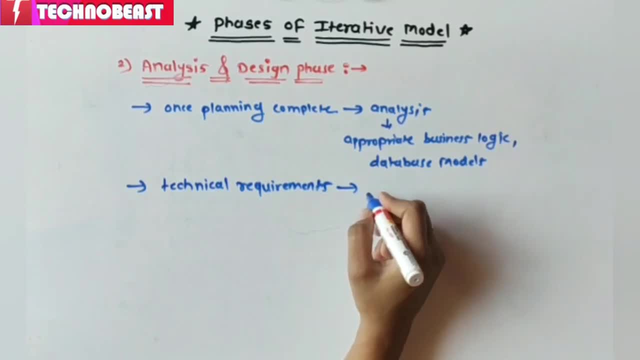 Which technical requirements, Like we can say that language database layer, services- okay, Languages database layer, and we can say that services and many more. These are the technical requirements we are going to be established here That will be utilized to introduce. 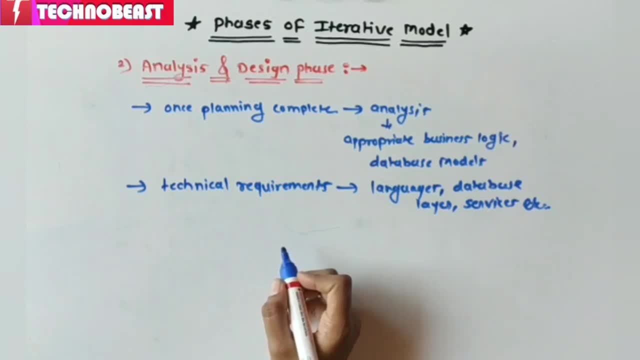 We have to meet The need to the analysis or analysis stage. okay Means these technical requirements we are establishing for meeting for meet the analysis stage. right Means: whatever we are going to decide to do in analysis phase will be decided with the help of these technical requirements. 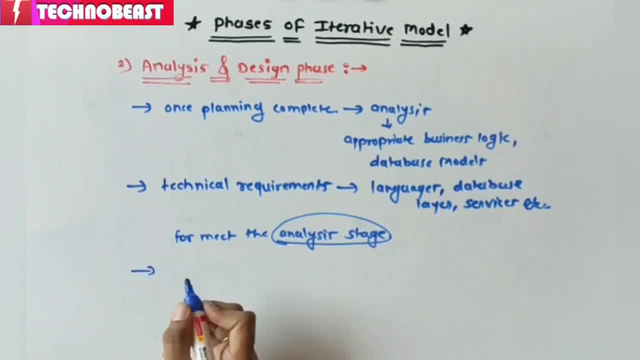 In this design phase, the software solutions. The software solution is prepared right Means here, the software solution is prepared right. The system design may be a new one or the extension of previous build. one Means here the technology or system design. we can say that here the system design. 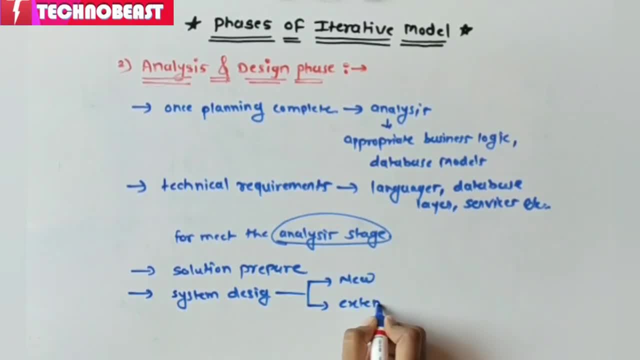 Either it will be a completely new Or it is a extension of our previous one That is already built model, or we can say that any project or designs okay To meet the necessary or necessity for this design of the project, okay. So these all are the happens inside the analysis and design phase. 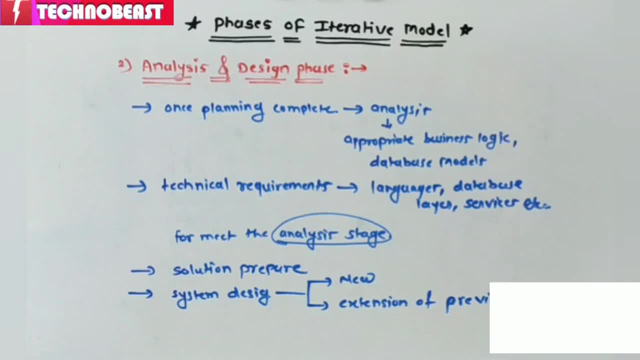 Means. once we have to complete our planning, Then we are moving towards the analysis part And in this we are deciding some appropriate business logics and database models which will be used inside the project. After that will be decide the designing of the project with the help of this technical requirements.